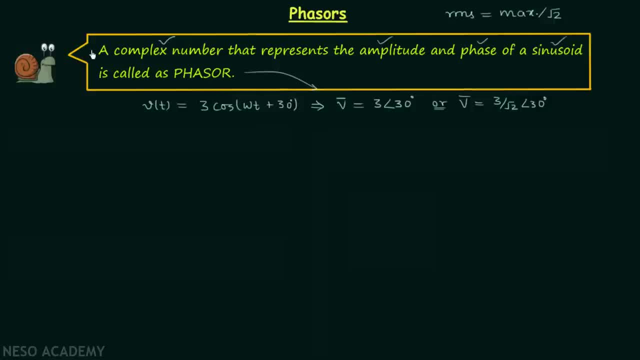 of complex numbers, because phasor is nothing but a complex number, And we will quickly arrive at a way of doing so. now, before we go further into details on phasors, we will movie to its basics, And before we go further into details on phasors, we will quickly revise. 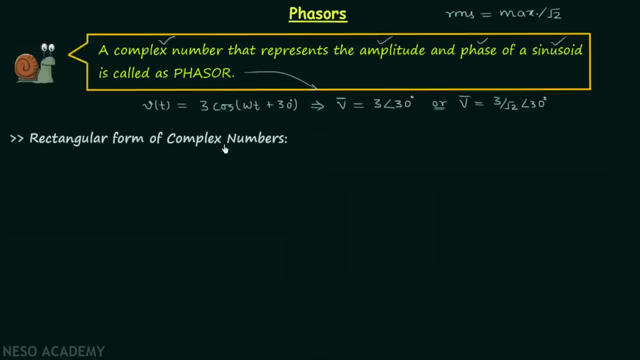 the basics of complex numbers. Now we are required to know. the basics of complex numbers will start with the rectangular form of complex numbers, And let us say that our complex number is represented by Z And we know it has two parts. The first part is known as the real. 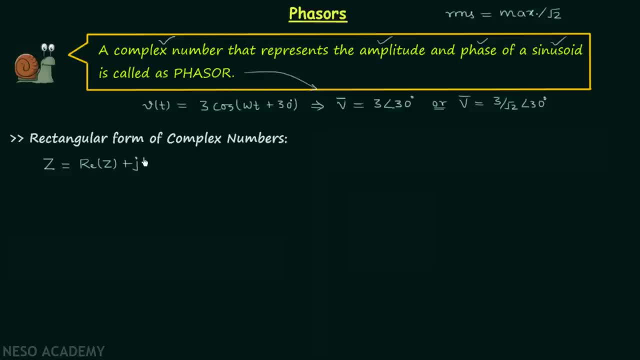 part of the complex number and the second part we call imaginary part of the complex number. And let us say that the real part of the complex number is equal to x and the imaginary part of the complex number is equal to y, and therefore we can say that our complex 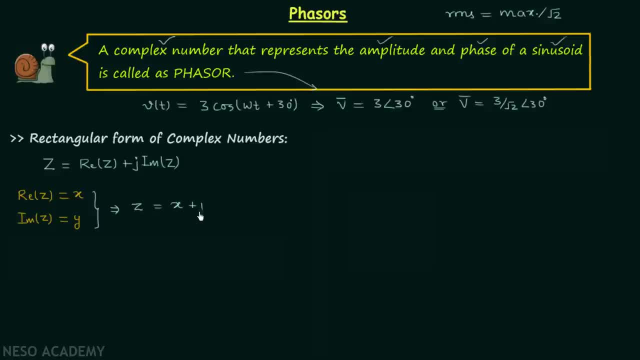 number Z is equal to x plus j, y, And we know j is equal to under root minus one, a. So this form we call as rectangular form of the complex number. and now we will talk about the polar and exponential forms of the complex number. The complex number z in polar form is written as r, which is the magnitude, with angle theta, which is the phase angle, and the exponential form of the complex number is equal to the magnitude multiplied to e power. 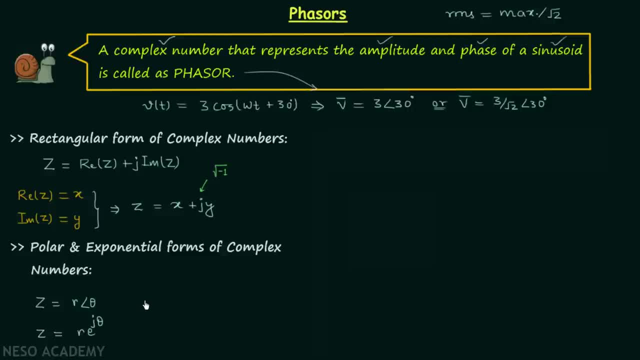 j, theta. and, as I told you, r is the magnitude of the complex number and theta is the phase of the complex number. And now we will find out the relation between polar and rectangular forms. That is, we will try to have r and theta when x and y are given, and we will try to have x and y when r and theta are given. And for this I 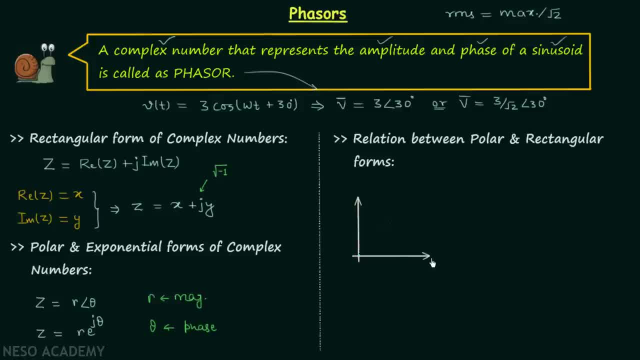 have taken the rectangular coordinate system. The x axis is for the real values of the complex number and the y axis is for the imaginary values of the complex number. And let us say that our complex number z is equal to x plus j, y in the rectangular form, And this means from origin to the value x on the real axis. 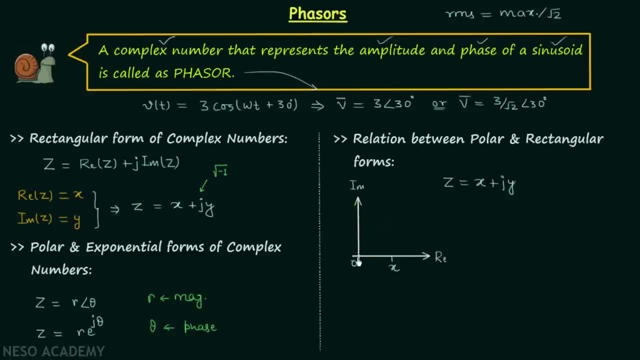 is our real part of the complex number and from origin to the value y on the imaginary axis is the imaginary part of the complex number And corresponding to x and y, we will have a point on the complex plane. And now we can visualize our complex number as a vector like this, And this vector will have the magnitude equal to r and 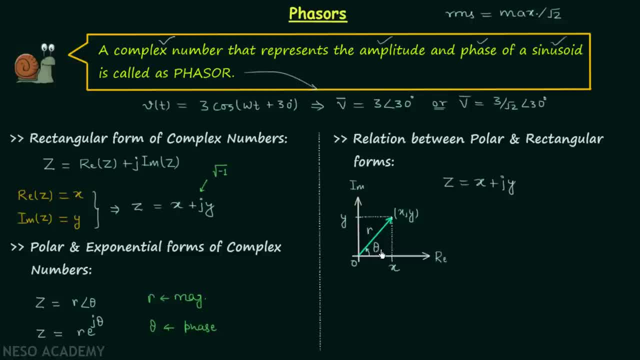 from origin to the value z and v is given, This line will make an angle equal to theta, which is the phase of the complex number. Now when you focus on this triangle, you will find r is the hypotenuse of the triangle and we know it is equal to under root. 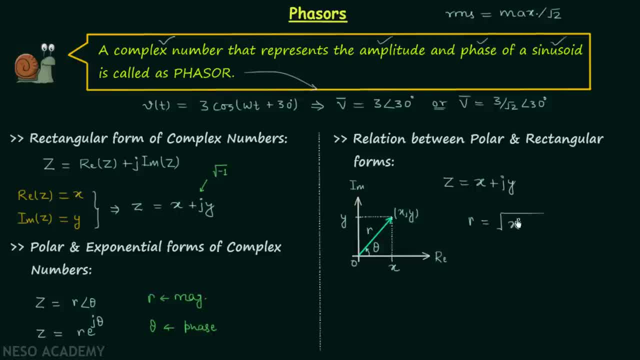 square of the base, which is x, plus square of the perpendicular, which is y. So if we have x and y, we can have r from this point on. So, identity of z productionающego, All of these are related To obtain the neue finite State. 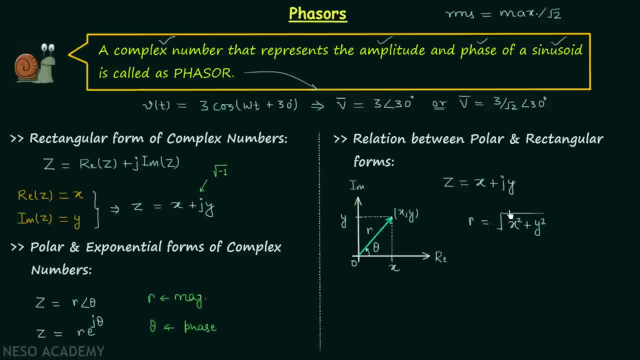 In this particular case, we can use ourillah. So that's it All. right now, that is enough, Let's do the whole system. particular result: And we know that the slope is equal to 10 theta and 10 theta will be. 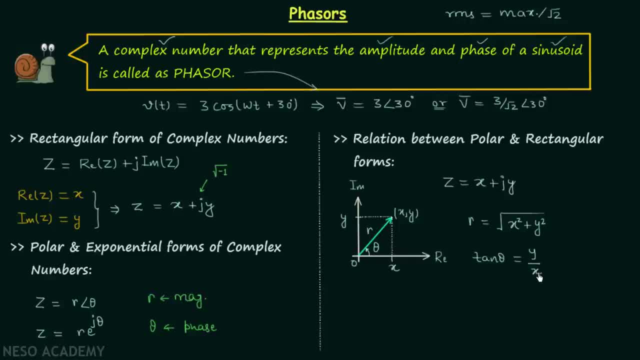 y over x, y over x. So from here we will have the phase angle theta equal to 10, inverse y over x. So if we know y and x, we can have theta as well. Now what if we know r and theta? 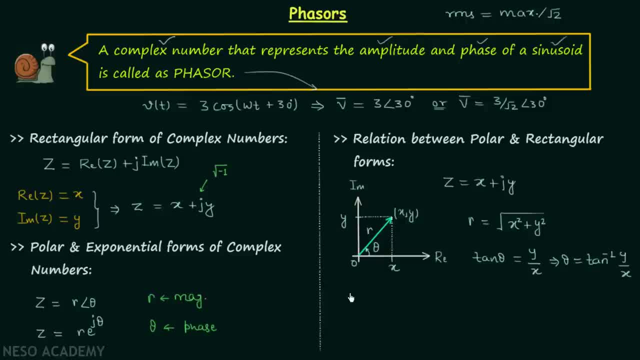 and we are interested in finding out y and x. Then you can see that cos theta in this triangle will be equal to x divided by r. So from here we will have the real part of the complex number equal to r multiplied to cos theta, And sine theta will be equal to. 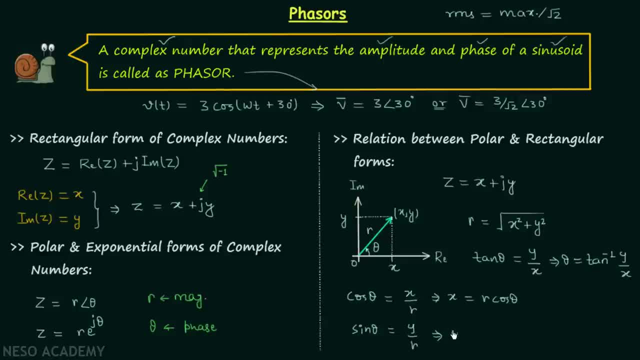 y over r. So we can say that the imaginary part is equal to r sine theta and therefore our complex number z will be equal to r cos theta plus j sine theta. Now we will continue with our discussion on phasors. The phasor representation is based. 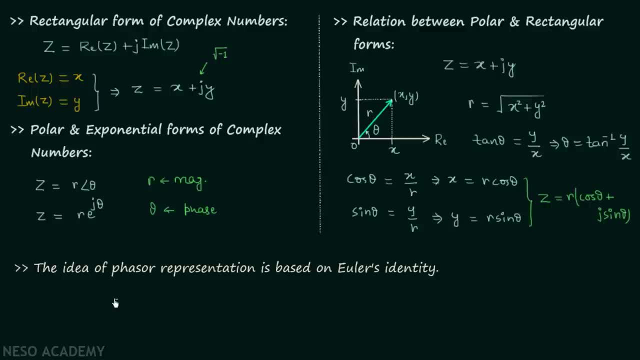 on Euler's identity, and we know the Euler's identity is e power j theta is equal to cos theta plus j sine theta. and when you compare the right hand side with this, you will find the real part of e power j theta is equal to cos theta. 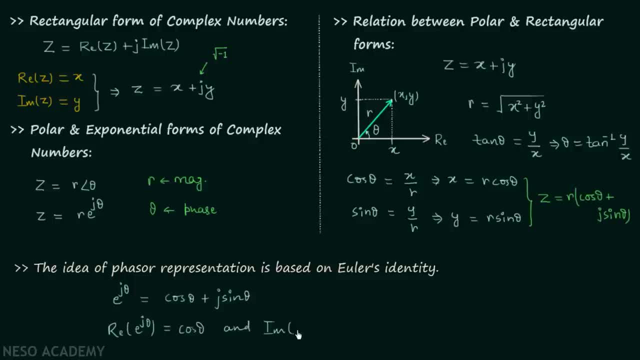 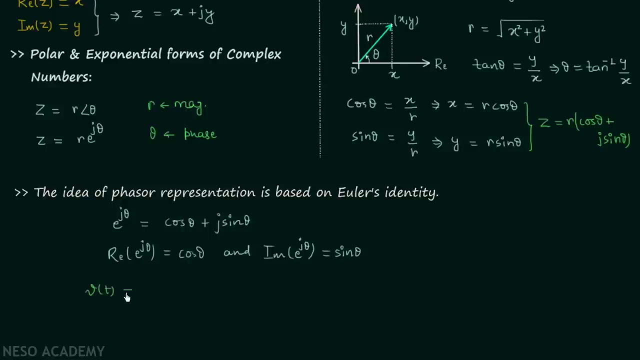 And the imaginary part of e power, j theta is equal to sine theta and let us say that the sinusoidal function we are having is Vt and it is equal to Vm cos omega t plus theta. Now compare Vm cos omega t plus theta with cos theta. you will find in place of theta. 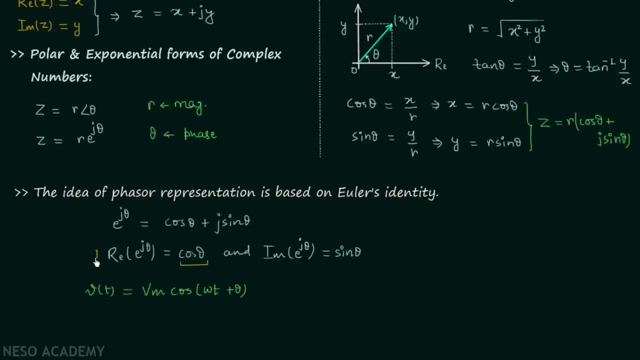 we have omega t plus theta, and here one is multiplied, so one is multiplied to cos theta, but here Vm is multiplied, so we will have Vm, real part of e power, j, omega t plus theta, equal to Vt. so we can write: Vt is equal to real part of Vm, e power, j, omega t plus theta. 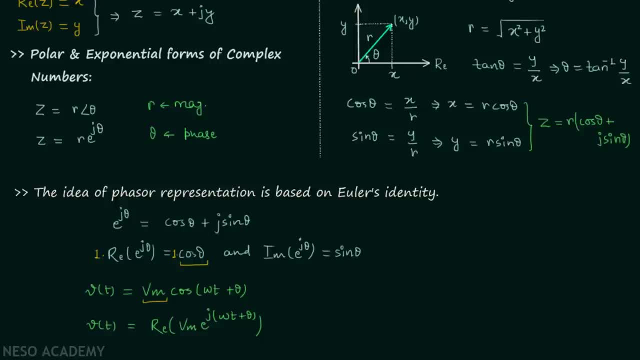 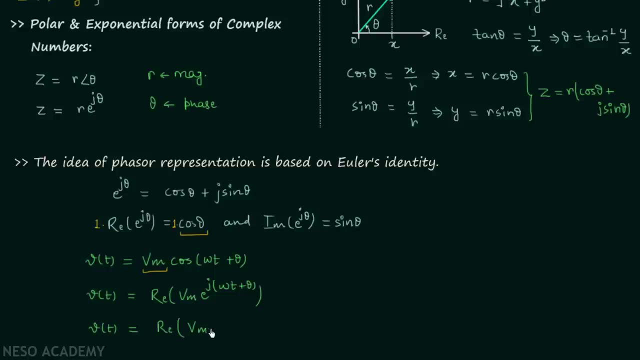 plus theta. Now we can further write Vt, equal to the real part of Vm. e power j, omega t multiplied to e power j theta. Now we will suppress this term: e power j, omega t, which is the time component. So here we are, suppressing the time. 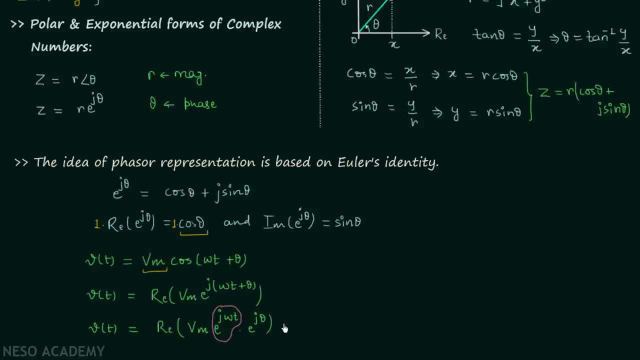 component and after suppressing the time component, we will have Vm, e, power, j, theta, and when you compare this with this, you will find Vm is the magnitude and theta is the phase. and this is the exponential form of the complex number which we call as the phasor, and we can represent phasor like this also: the 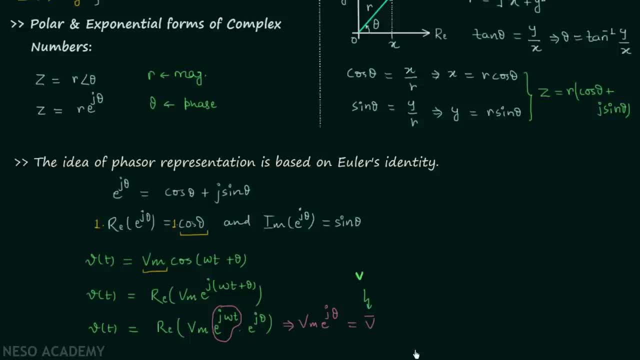 upper case and bold Vm, And we usually write our phasor in the polar form, which is Vm, with the phase angle. So now it is clear that V phasor is the phasor of sinusoid Vt and it is a. 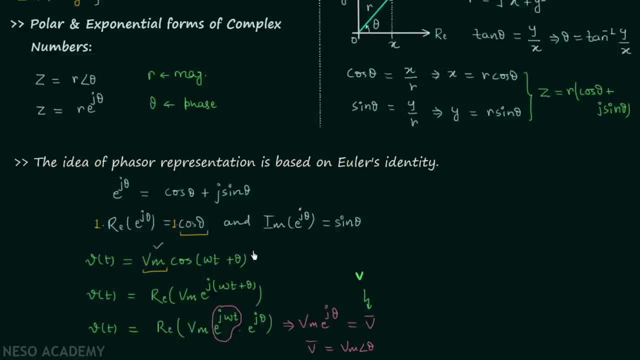 complex number representing the amplitude and phase of sinusoid Vt. and we are getting this complex number by suppressing the time component and therefore we can say that a phasor of sinusoid Vt is the phase of sinusoid Vt and therefore we can say that a 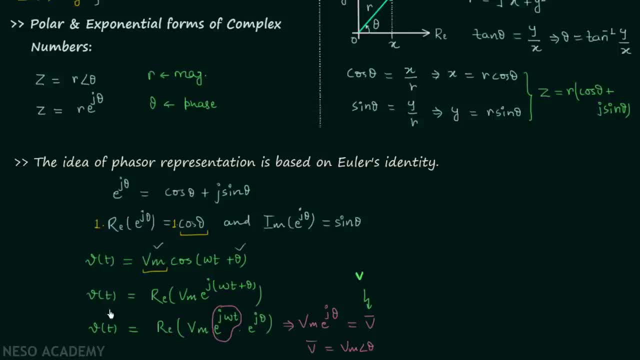 phasor is the mathematical equivalent of a sinusoid when the time dependence is dropped and therefore Vt is a time dependent quantity but V phasor is a time independent quantity and if you have the sinusoid, Vm sine omega, t plus theta in, 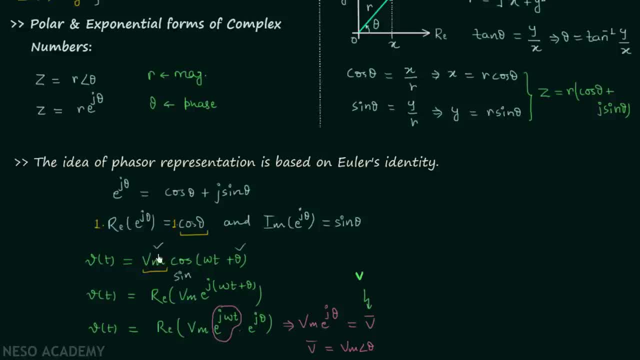 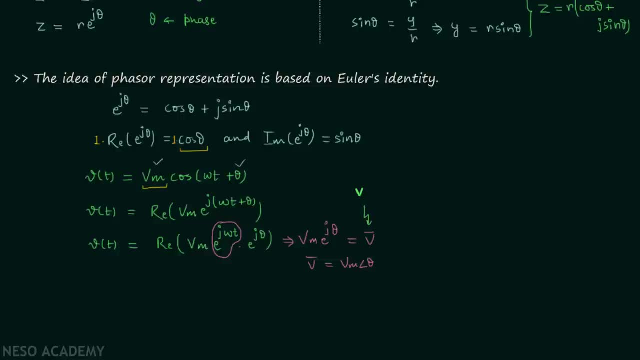 place of cos. if you have sine, then also the phasor is going to be same. now I will take two phasors and I will try to plot them in the same complex plane. this is our real axis and this one is our imaginary axis, and the first phasor is V phasor and it is equal. 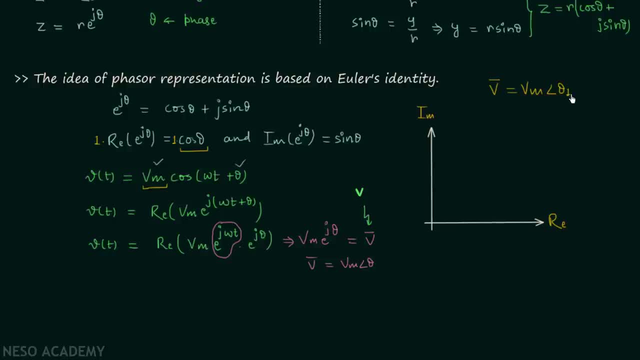 to Vm, angle theta 1, and the second phasor is I phasor and it is equal to I M angle negative of theta 2.. We will first plot V phasor. We will have a vector like this with magnitude equal to Vm, and it will 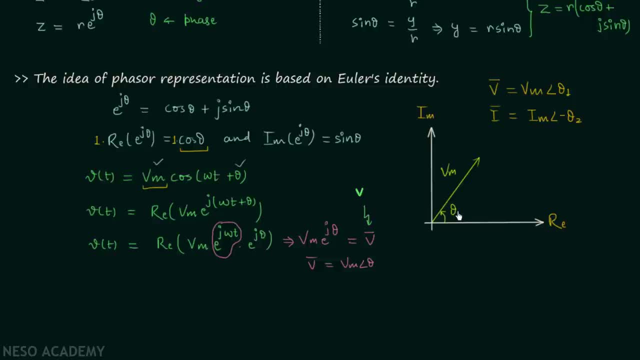 make an angle equal to theta 1 in anticlockwise direction with respect to the real axis. We are done with this phasor. Now we will plot this phasor. We will have a vector making angle theta 2, but in the clockwise direction with respect to the real axis. Why? Because here we 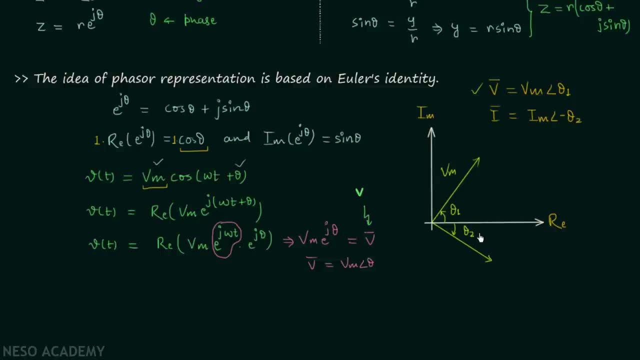 have negative of theta 2 and we know angle measured in clockwise direction is negative and angle measured in anticlockwise direction is positive and this will have the magnitude equal to I- M. So this vector is our phasor, V phasor, and this vector is our phasor, I phasor. and there is one.